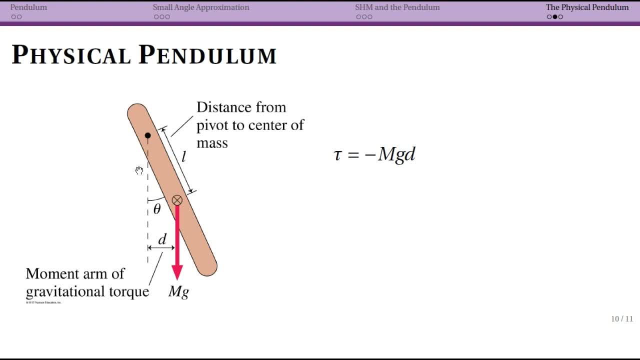 rotation and thinking about torque. right that we're talking about a pivot point here and the center of mass some distance away, so that looks like torque. Now remember that there are different ways of thinking about torque, and one was thinking about the distance that is perpendicular to your force between where the force is applied and the pivot point. So in this case, the torque. 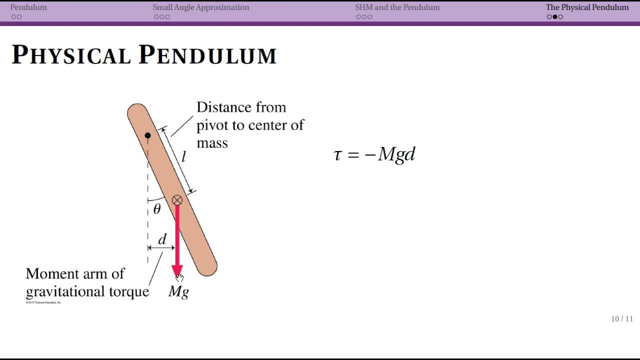 from the force of gravity acting at the center of mass is equal to mg, where that's the force of gravity your force times d, where that is your moment arm. So the distance in the x direction from your center of mass and the- remember that the minus sign is coming from the coordinate- 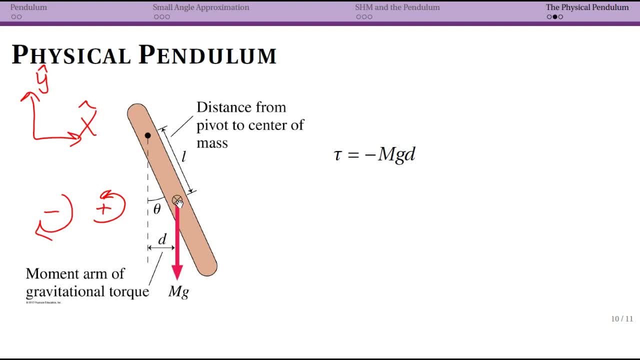 definition that d is a positive, So that's the value here, because your center of mass is to the right of your pivot point. But if you think about which way gravity is then going to make this object rotate, it's clockwise, and clockwise is negative, So that's why there's a minus sign here. So now let's. 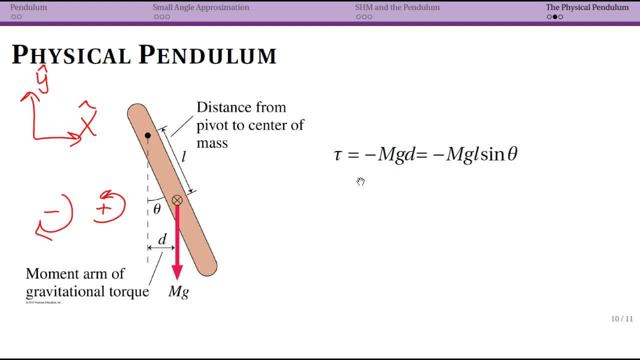 expand that in terms of theta. So d is just going to be this length here, the distance from the pivot to center of mass times sine theta. And the reason we want to do that is that as it rotates, d is going to be changing. It's also going to become negative when this whole object 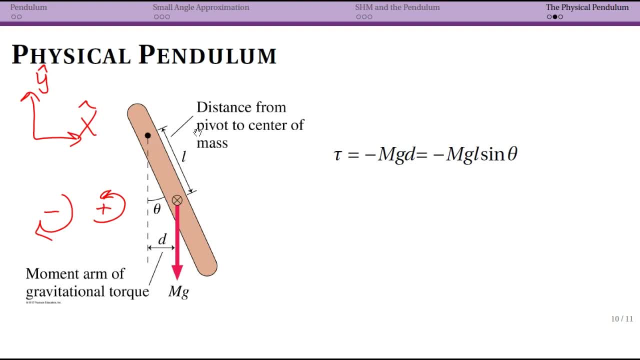 has rotated to be on the other side, But L is fixed, L is constant, So we can now express theta as impacting our torque. So once again we notice that we have a sine theta here. This is possibly going to be a problem, But we can now use the small angle approximation. 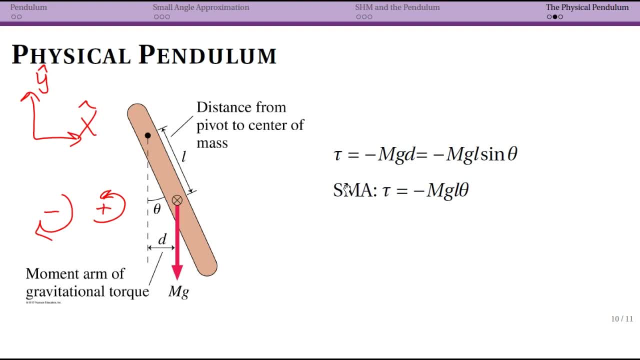 which I'm. as a physicist, I make really bad acronyms, So small angle approximation, you might think should be SAA, but now I'm going to call it apparently SMA. So what we've done is said that sine theta is approximately equal to theta. So keep in mind that if I'm doing that, 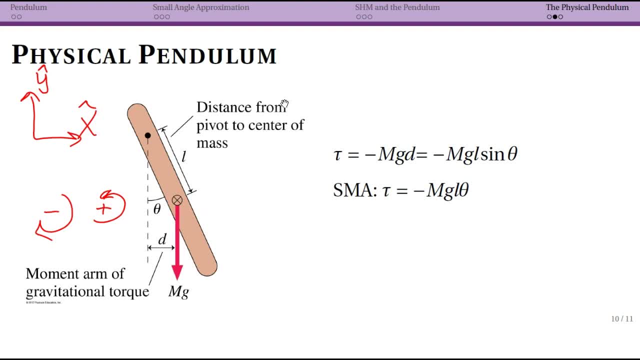 I can only be talking about small oscillations, not big swings here. So then, what? Now? remember that torque is related to moments of inertia. I and alpha, our angular acceleration, And angular acceleration is also going to be defined as the second derivative of angle, with respect, 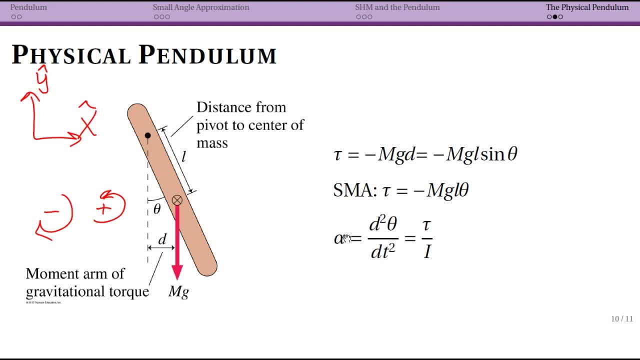 to time. So now what you see is I have an angular acceleration that I can relate back to torque. Right here we're not talking about forces, because we're talking about rotation, So I haven't defined what my moments of inertia is. i, that's OK, Because we're talking about 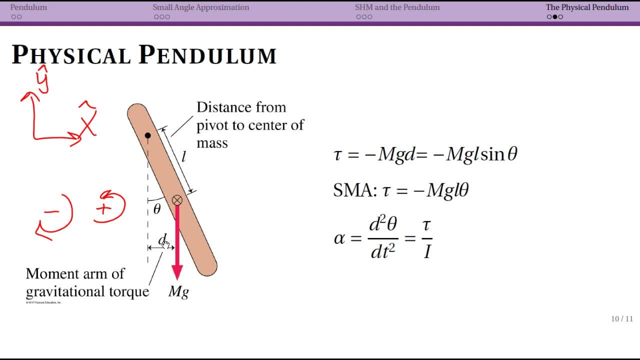 this in general. This might look like a specific type of object, but it could be a much more complicated object. This is how you would model, for instance, people perhaps swinging on a UV colour of some young person with white hair. I might see that you might have When you're right near this time, if this goes about time. 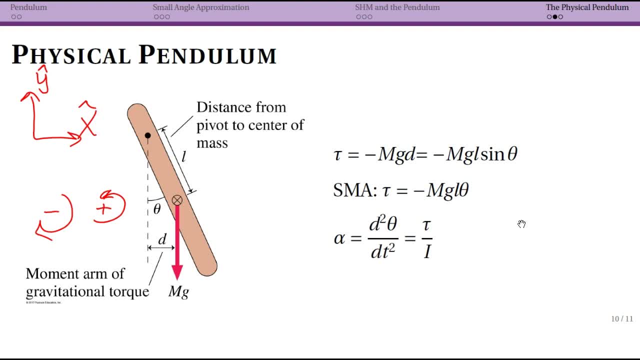 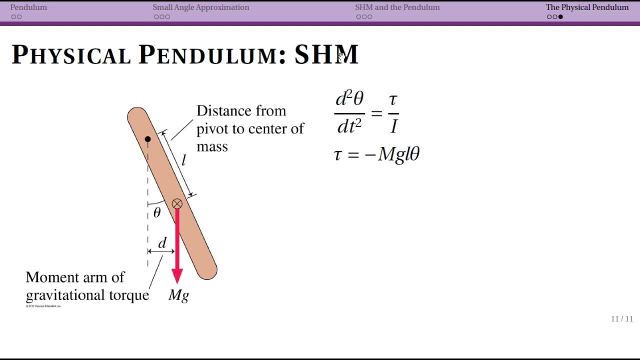 people swing at this stretch of time, or the speed and direction. This could be a much more complicated object. This is about this angle: uh, one of those hanging wooden uh chairs or something so there's could be have a really complicated moment of inertia. so let's try to get this to the form of simple, harmonic motion. 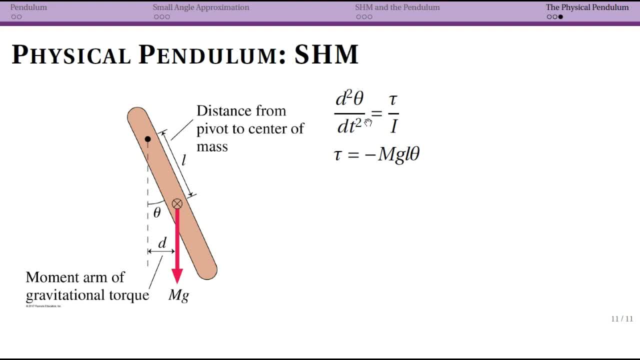 i've said that my angular acceleration, which is my second derivative, is equal to tau torque over moment of inertia, and i've said my torque, as long as i'm dealing with small angles, relates to negative force of gravity. the length of between my center of mass and the pivot point. 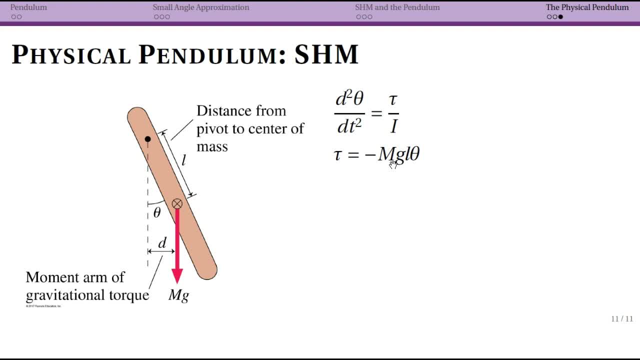 and then theta. so the first thing you should ask yourself is: do i have a linear restoring force? if you do, it can be modeled as simple harmonic motion. if you don't, it cannot be. so the linear restoring force is here because this is your position and there's. it depends on theta. it 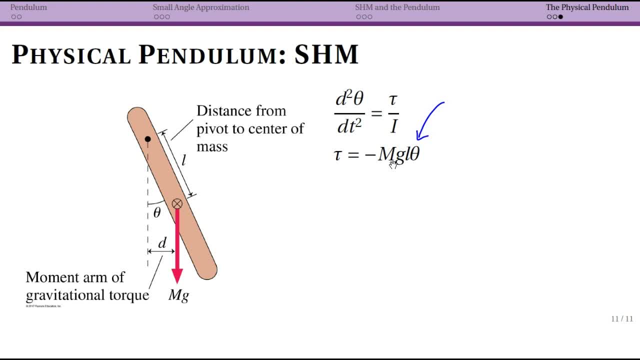 doesn't depend on square root of theta or theta squared, and so you have a force that depends on your position. it's restoring because you have a minus sign and then there's just some proportionality of three constants multiplied together, so this looks like a linear restoring force. we then plug it in for for tau, and we're left with this form. 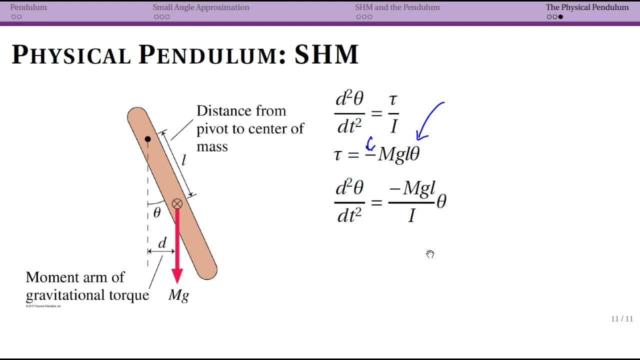 now again. your goal here is to recognize when you know how to solve a differential equation by writing down what the solution is. i have the second derivative of a coordinate, in this case theta with respect to tau. and then i have the second derivative of a coordinate, in this case: 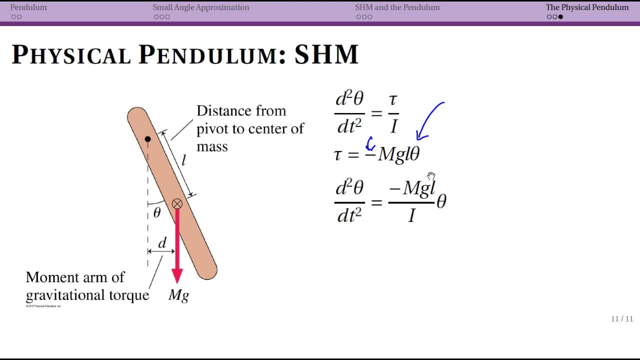 theta with respect to tau. and then i have the second derivative of a coordinate, in this case time. it equals to minus. that's good. a group of constants times theta itself. this is the form you need. right that the form we talked about before was, for instance, d squared of u over dt squared. 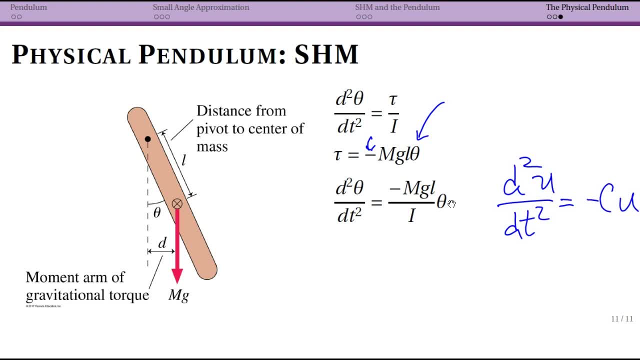 equals negative some constant u. that's exactly what i have, where u is theta and the c is mgl over i. so what that means is this is going to be solved with our sinusoidal form, where again, i could express that in terms of arc length if i wanted. here i'm going to do it in terms of theta, since that's what i started with. 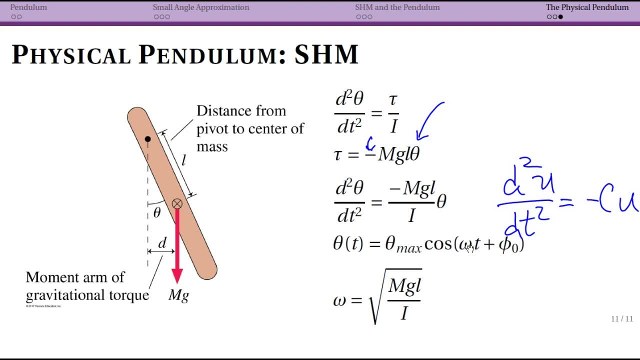 so we have a maximum angle that it swings to, we have our angular frequency and our phase constant. again, remember, this isn't a physical angle, this is a mathematical angle of where it is in the sinusoidal motion and this is going to be determined by initial conditions. omega is 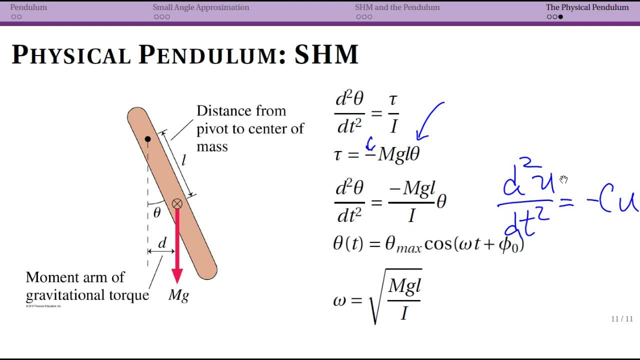 now equal to just the square root of all this nonsense. keep in mind, the minus sign is always out front. don't take a square root of a minus sign, because then you get imaginary numbers and that's bad in physics class. so it depends on the mass of the object, times, gravitational constant times, the. 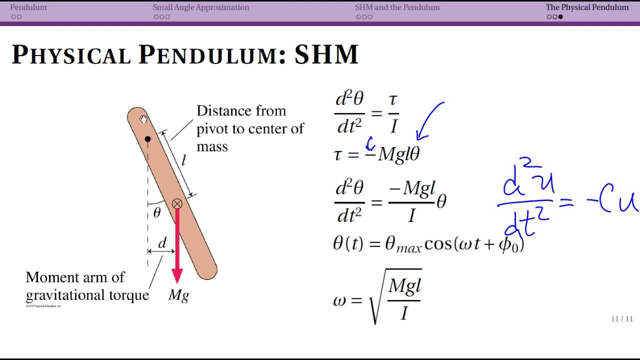 length again between the pivot point and your center of mass, not the length of the entire object divided by the moment of inertia. now, one caveat here is that this moment of inertia depends on the shape, but is usually the moment of inertia, and the moment of inertia is the moment of inertia. 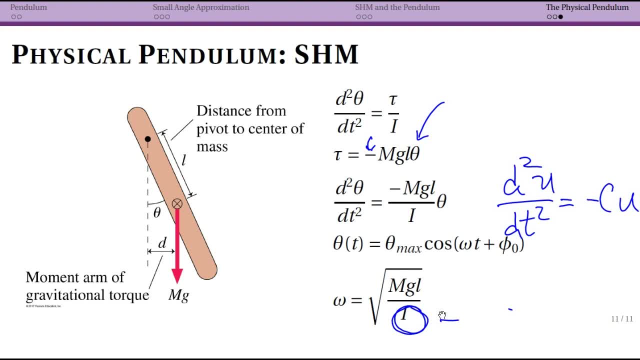 so we're going to have the form of some constant right, so some numerical constant times, m times, for instance. some length squared or radius squared m always appears in the moment of inertia, and so because of that, you actually are going to have m cancel on top with that. so really, your moment of 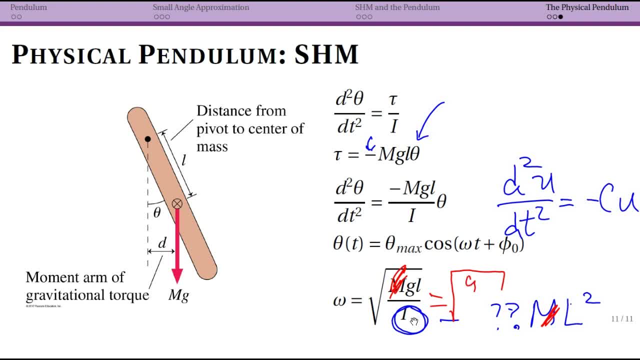 inertia is going to be g over g times l and that's going to be the moment of inertia and that's going to be l times some sort of numerical value and again l squared, where this is a different l. maybe it's a radius, but some sort of length that 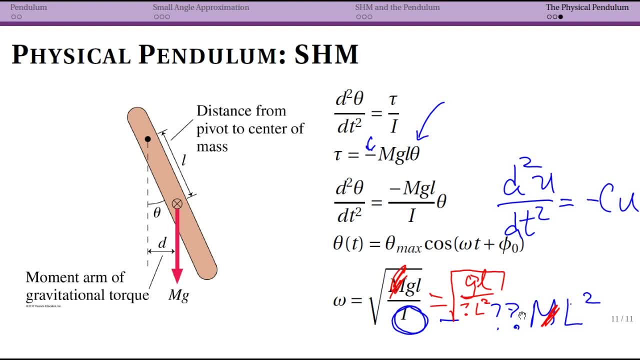 describes your object. so mass does cancel out, but that's because mass is embedded within the moment of inertia. so, again, the physical pendulum, as long as we're talking about a small angle of motion, again, is going to have simple harmonic motion because the force of gravity acting not at the